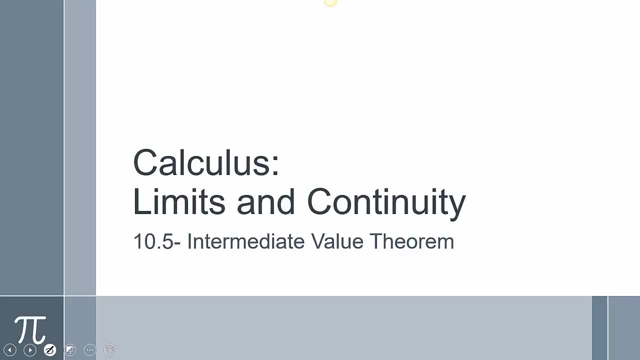 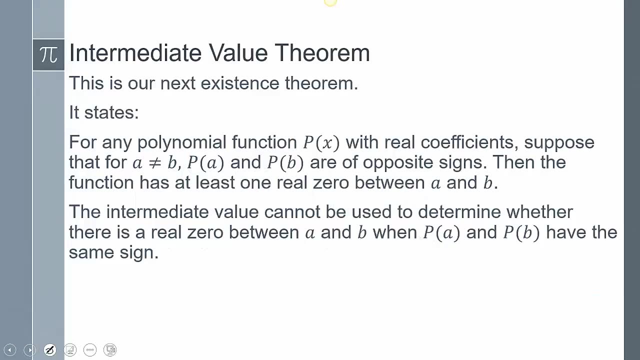 Today is 10-5.. I'm going to look at the intermediate value theorem. and we're still in the unit of limit and continuity. So the intermediate value theorem is our second existence theorem and here's the definition It states for any polynomial function with real coefficients. suppose that if a doesn't equal b, 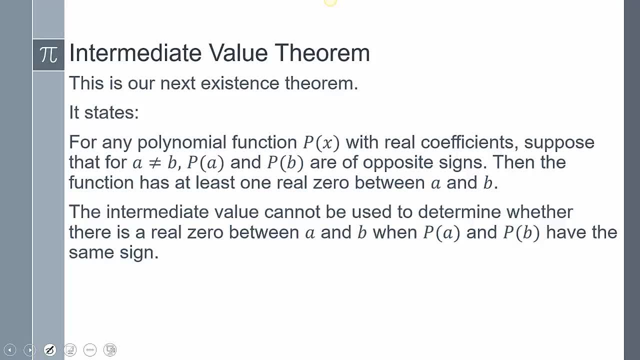 so your two x values can't be the same and p of a and p of b are of opposite signs, meaning one's positive and one's negative, then the function has at least one real zero between those two x values. Now remember, the intermediate value cannot be used to determine whether there is a real zero between a and b. 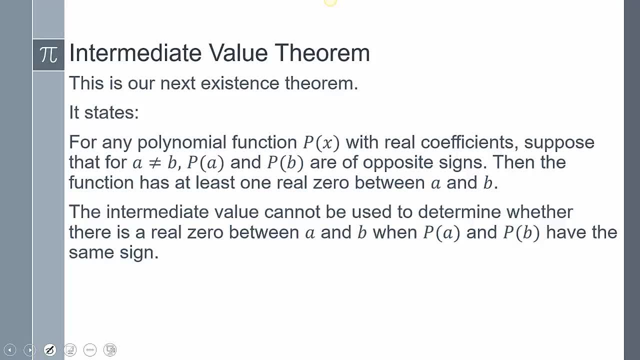 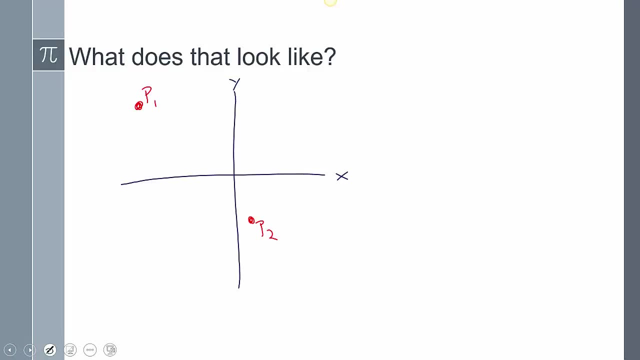 when p of a and p of b have the same sign. So let's unpack this just a little bit and then we'll kind of practice to show you what it means by the definition. So what does it look like? Well, if we have our x or y graph here and we have two points, 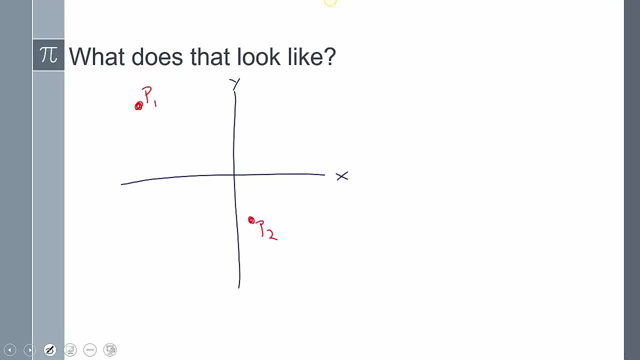 what it's saying is that if one is positive, so in this instance this one is positive and then one is negative. in that instance that's negative. it has to cross the x-axis. There has to be a zero in between there. 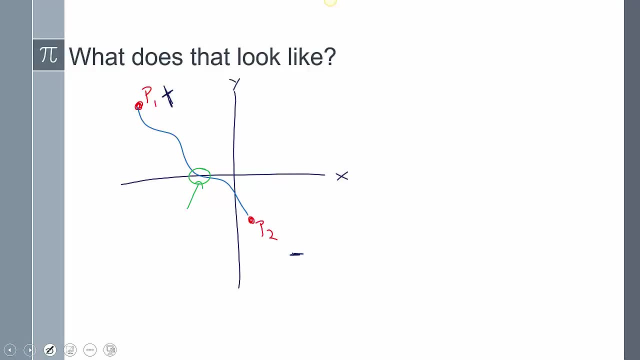 There's no other way to do it, because our function is continuous, And so the intermediate value theorem just says that within that interval you know that it's a real zero. So if we have our x or y graph here and we have two points, 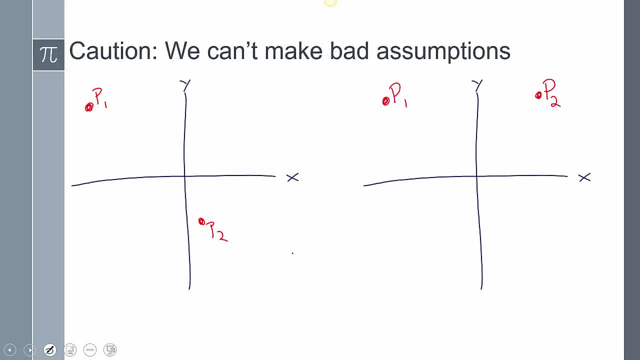 there has to be a zero in between there, But it's at least going to cross the x-axis. once Now we have to be careful of a few assumptions about the intermediate value theorem. So we have to be careful about these. The first assumption is: some of us think: well, if it crosses, there's only one zero. 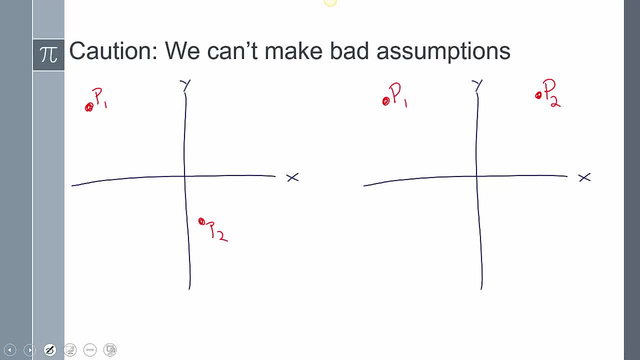 And that's not true. The definition says at least one zero, And what I mean is your function can do this. Well, this is positive, this is negative, and so, if you noticed, it crossed a bunch of times, definitely more than once. 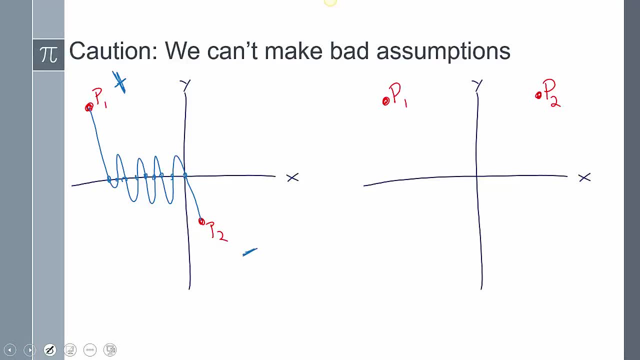 So we have to be careful about that. You can't say there is one zero, You just know there's at least one zero. The other bad assumption is, when the signs are both positive or both negative, Sometimes we assume: oh, there is no zero between there. 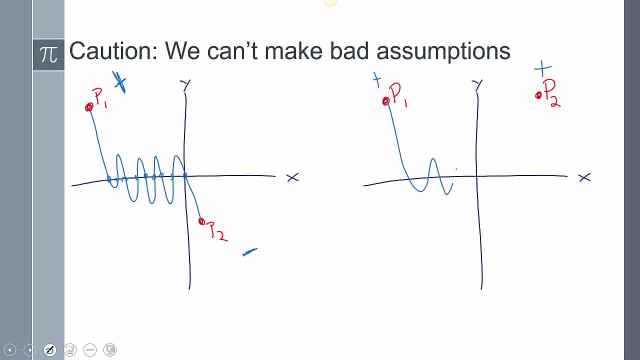 and that's also a negative. And that's also a false assumption, because your graph can do its thing and then go back up into the positive direction. in this instance, But notice- it crossed the x-axis a bunch of times in between, but yet they're both positive. 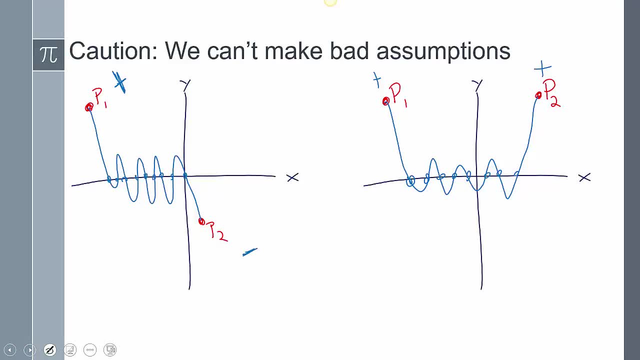 So just remember, when the signs are different, there could be more than one zero in between. We just know there's at least one Second if they're both positive or both negative. you can't tell, You can't assume that there aren't any. 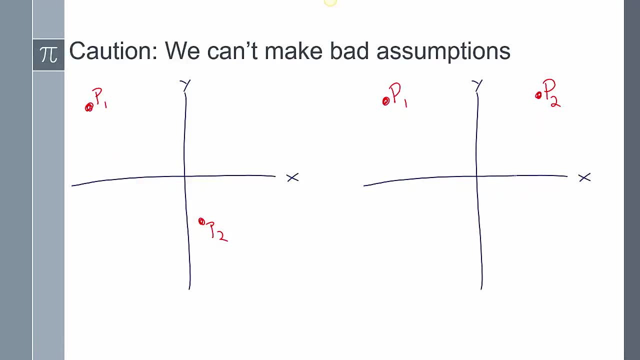 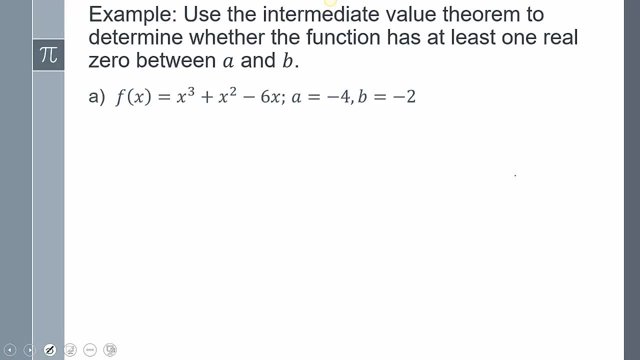 We just may have to do other things to try and figure that out. So here's a couple of examples. It says: use the intermediate value theorem to determine whether the function has at least one real zero between a and b. So we have to evaluate. 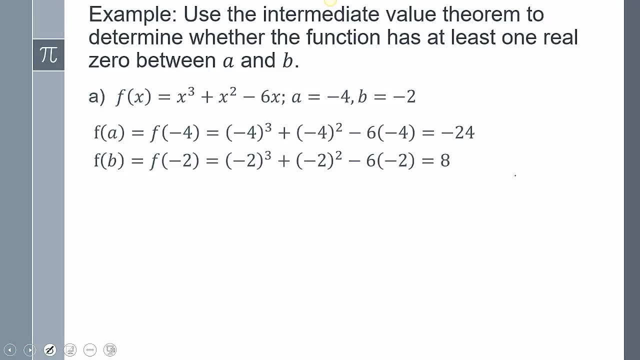 So I plug in negative 4, and I plug in negative 2, and I simplify it, And so I got negative 24 and 8.. Well, since the signs are different, I can conclude that at least one zero exists between a and b. 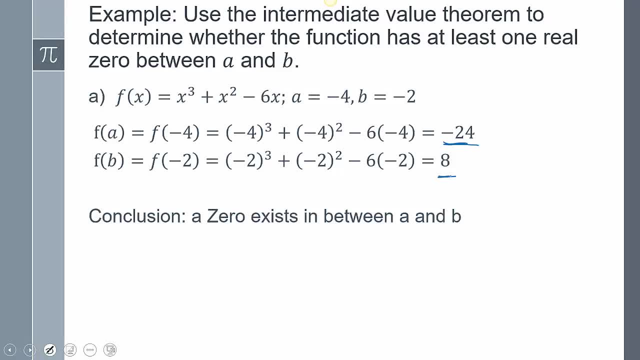 It could be 2.. It could be 3. But I know at least a zero exists between a and b. What if I chose the interval negative 1 and 3?? If I plug those in, this is positive and this is positive. 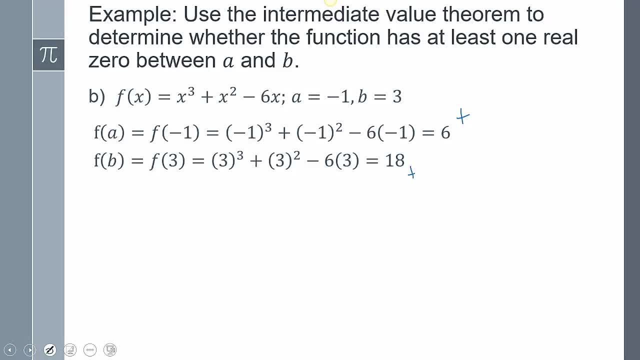 Now remember, we cannot conclude and say, oh, there's nothing in between. We can only say that we can't with this information. we just don't know, Right, There could be a zero in between, but right now, with this information, 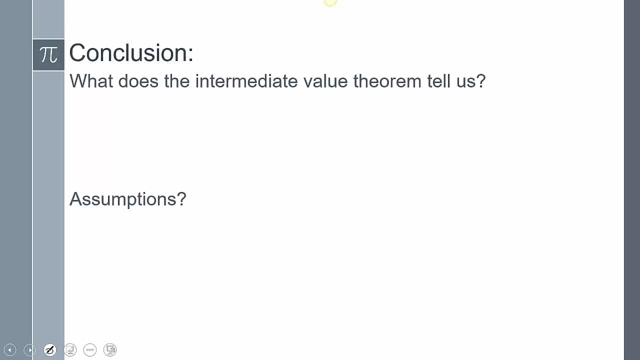 we just don't know if there is one or not. Now let's conclude the lesson. Now, what does the intermediate value theorem tell us? Well, it says that for two different x values, if one of the y values is negative and one of the y values is positive,